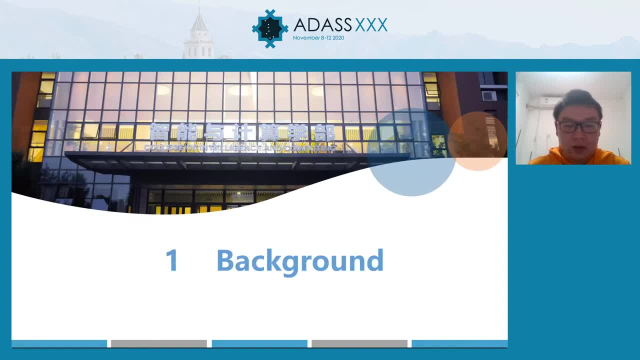 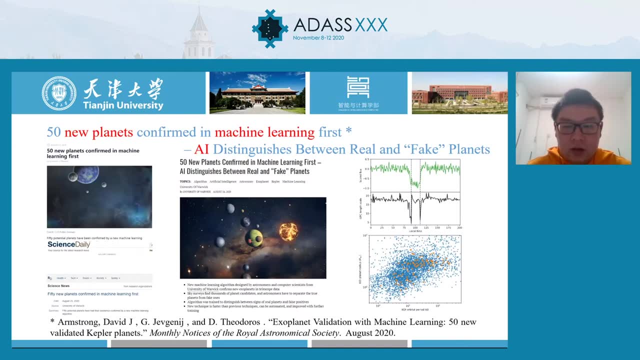 Okay, let's move to the first part: background. Recently, news has reported that 15 new plans confirmed in MASH learning. First, AI-distinguished data. All right, we will focus on a new and very important part of our work today, which is: how do you figure out the matching between real and fake plants? 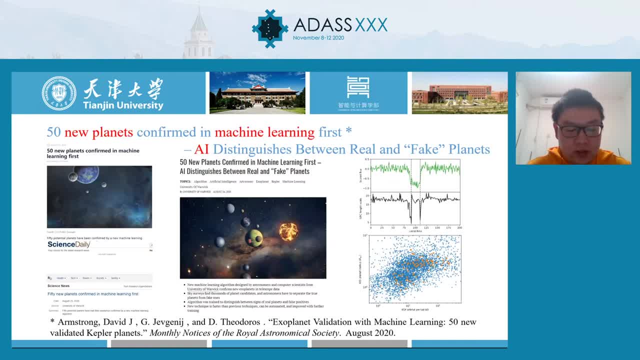 And the algorithm can upgrade 50 capillary contaminated plants to real plants across the threshold of planetary verification. This technique will hopefully be applied to large contaminated samples from current and future missions, such as test TSS. Recently, an advantage in the technique has provided adjusted efficiency, and it also increased the performance of the data that we use as a part of the project's development. 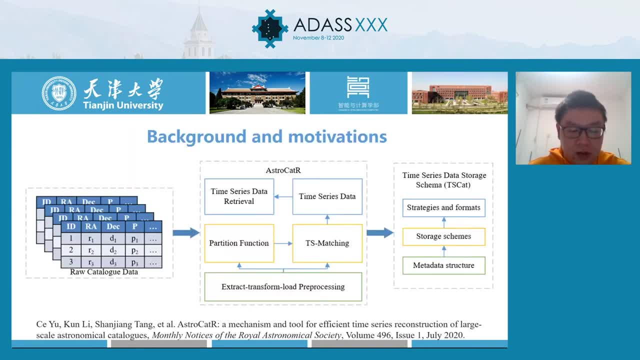 especially for testing energy, provided an enormous wealth of data for time domain astronomy. However, the organization of catalogs is inappropriate for time domain astronomy research because the time series information of each celestial object is indirect. To provide a large data sample for AI-based light cover analysis, astronomical catalogs need to be converted to time series data size. 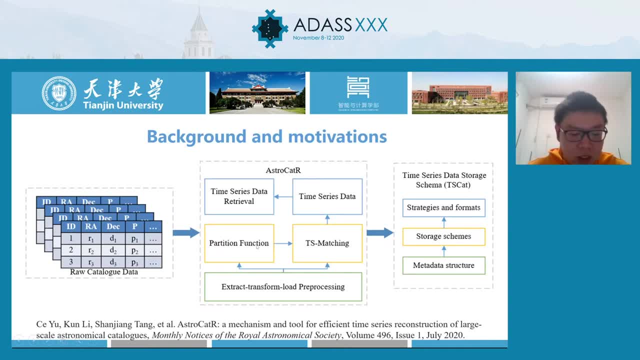 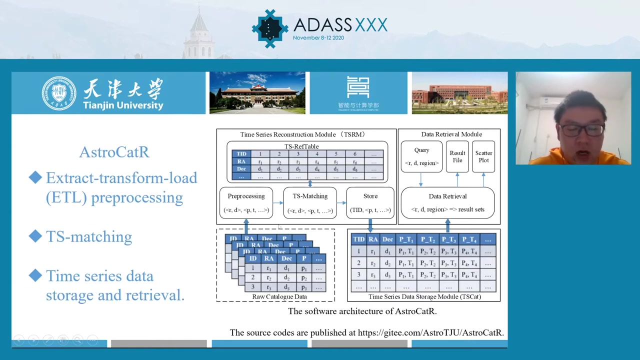 and the processing are shown in this figure. The intermediate time series data construction tool has been designed and implemented, called AstroCod-R. Now I will give a brief introduction of it. As the figure shows, AstroCod-R consists of ETL processing, TS matching time series data. 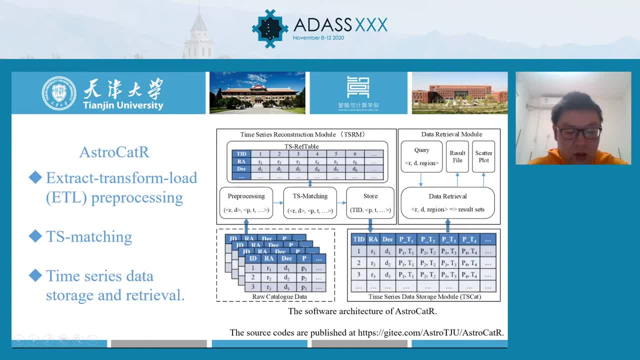 storage and retrieval. The astronomical catalogs are transformed into Skyrim fields and the load is balanced through the partition function. TS matching is a special design for time series data reduction based on the data. The ETL processing is a special design for time series data reduction based on the data. 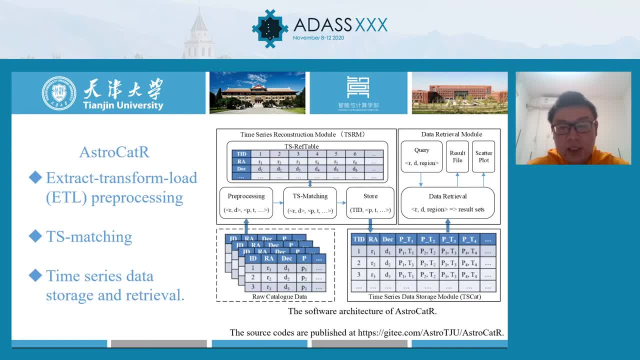 The ETL processing is a special design for time series data reduction based on the data. The ETL processing is a special design for time series data reduction based on the data Crossmatched. the matching calculation is performed to generate time series data size by the overlapped indexing method and in-memory reference table. 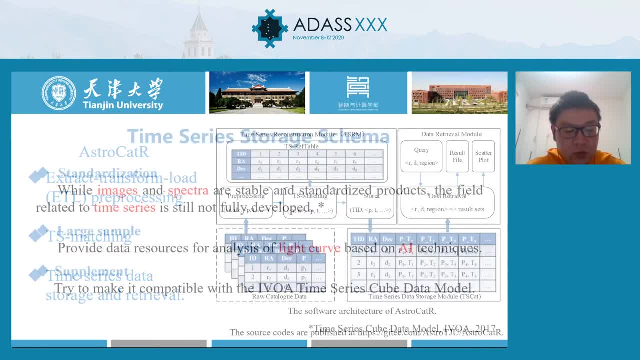 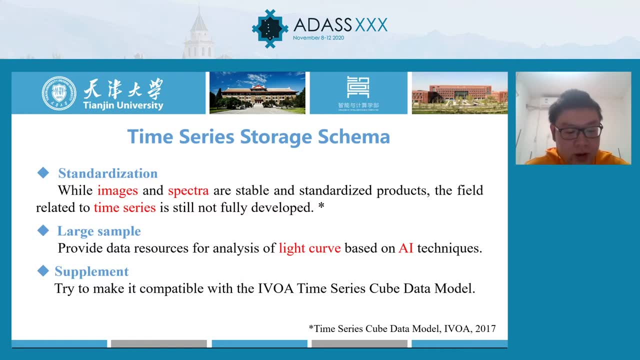 Currently, there are a variety of standards for most data sizes in the application of AI techniques. in light cover analysis, Whale Imagens and Spectra are steadily growing. Investors are restricting their time series data consumption to 120 nm of time. stable and standardized products: the field related to time series is still not fully developed. 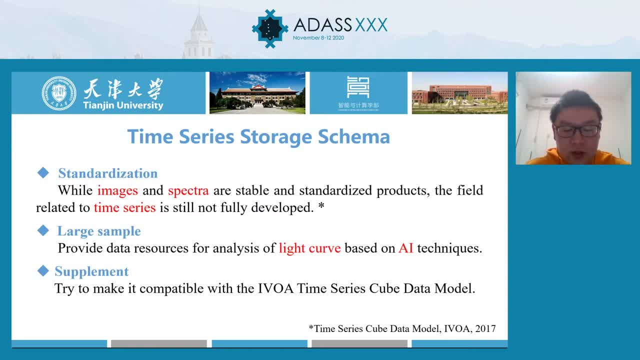 recommendation: unified light cover release standard needs to be proposed for analyzed of time series data based on the ai techniques. we focus on the challenges in time series made: data structure, storage schemas, strategy and formats of exposition generally. time series data exposition formats needs to spot csv fees and view table. we will try to make it compatible. 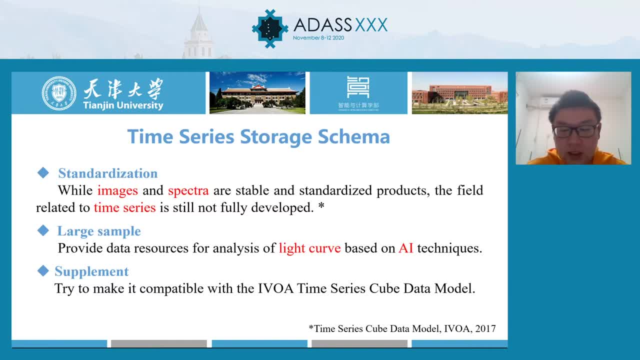 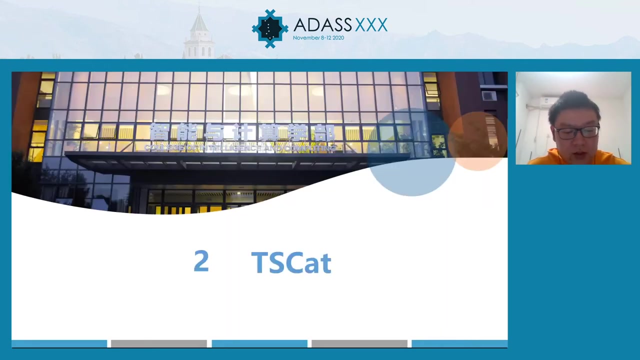 with iboa time series curved data models. we propose a storage schema named ts cat, which is a special design for storing time series data and it can conducive to time series data retrieval demands are for provenance, link linkage and life cover analysis. next i will give you a introduction of ts cat. 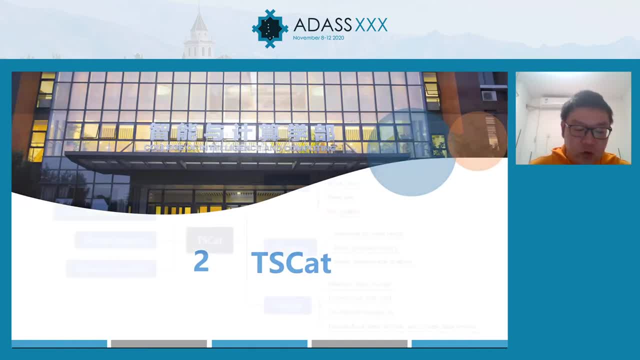 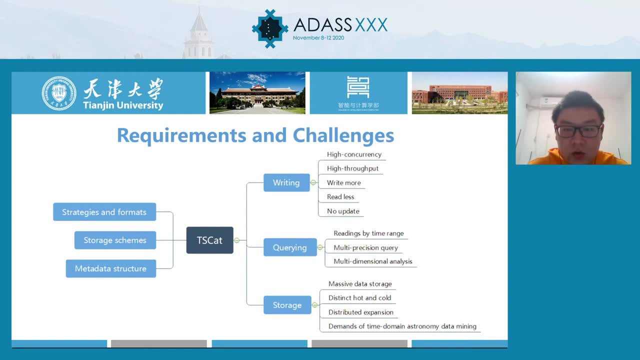 we will start it by describing the characteristics of astronomical time series data retrieval. we will begin with the basic requirement for time series data in switch domains: writing, querying and storage. the basic- the base basic requirements for time series data storage and management include: spotter for high currencies. writing high throughput, super support, uh writing. 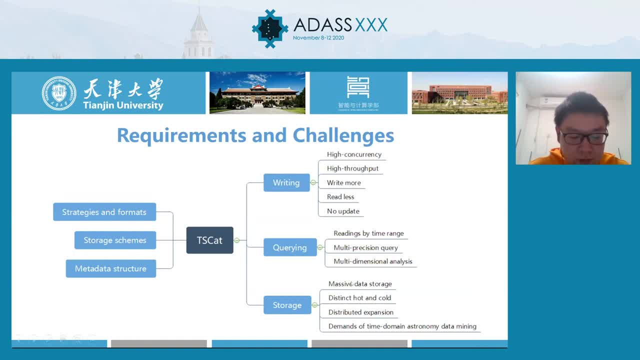 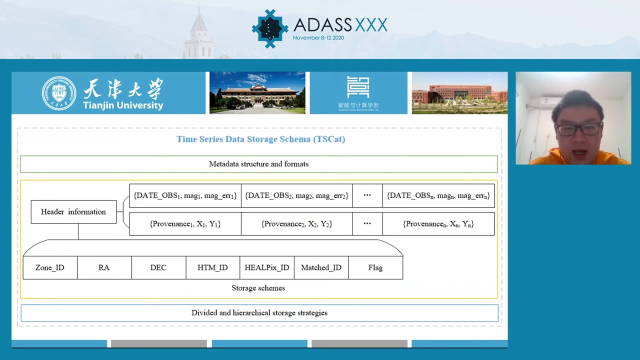 and massive massive data storage, aggregate query and distributed expansion. Additionally, the characteristics of different much learning algorithm and deep learning models are taken into account to meet the needs of time domain, astronomy, data manner as much as possible. This figure shows the overall architecture of TS-CAD. 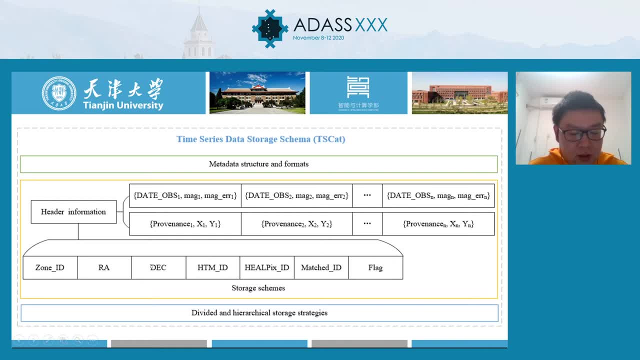 The common information for the same celestial objects need to be stored only once at the beginning and followed by time series tuples. This figure shows a sample of celestial objects in TS-CAD storage schema And the head information includes zoom ID, RA, DEC, HTM ID, HAPS ID, matched ID and flag. 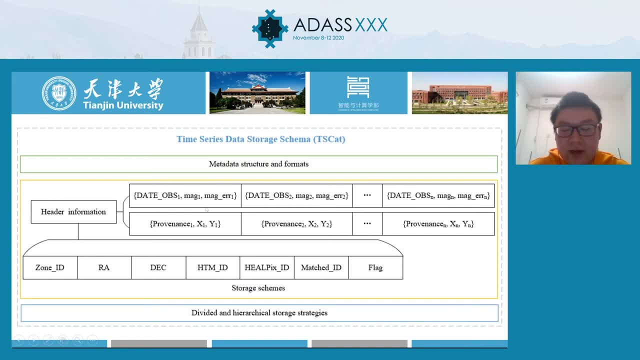 And the time series tuples are currently divided into two groups: One for AI technique analysis. the other group is used for tracking sub images To make the best use of storage space. the time series tuples used in light cover analysis only records observational times. 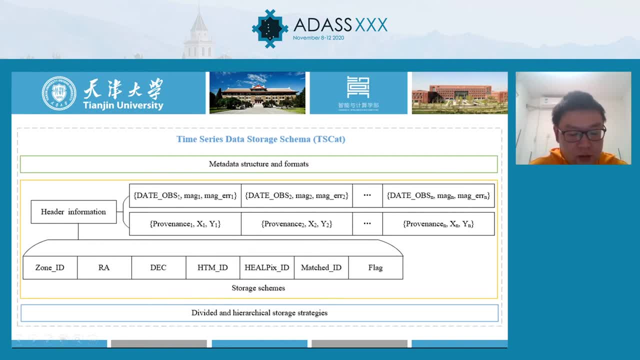 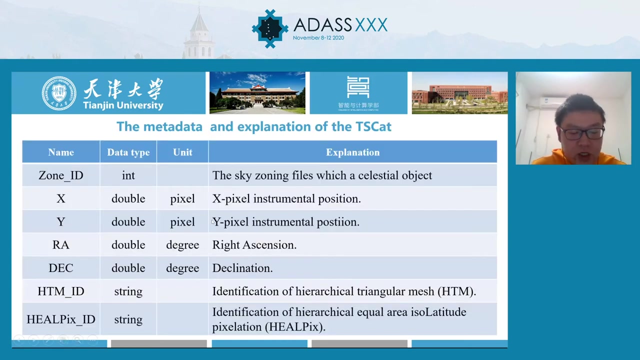 and magnitude information, And specifically date of observation, magnitude and magnitude error, the tuple use for trinking, sub images, directors and provenance information, Such as a provenance X and Y. We focus on the definition of meta data and topics: topics for time series, data such as original. 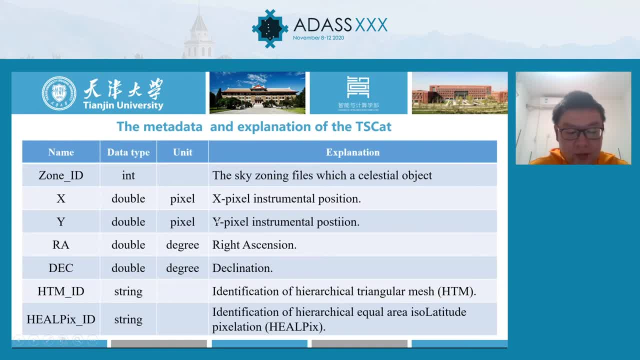 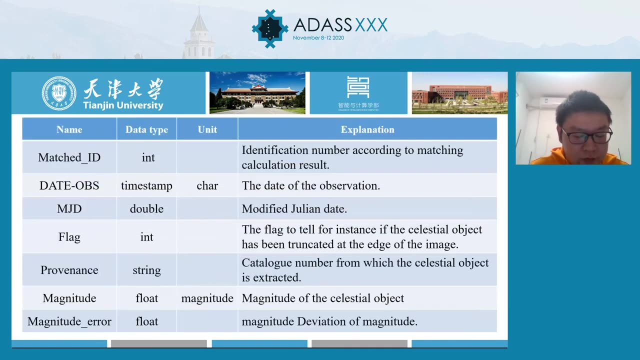 has a light cover on the sides and the shrinking sub-imagines for every individual point of light cover. This table shows the list of the made data and the explanation for time-series data. The divided and the hierarchical storage are designed to spot the light cover retrieval. 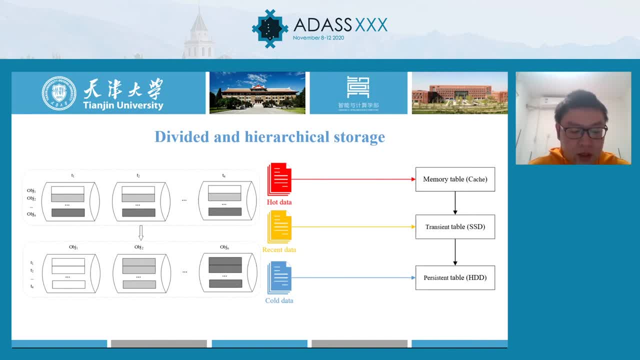 and analysis. In the divide storage schemas, the data of the same selection is changed from being stored in different areas to center centralized storage in the same area and divided according to its observational time. There are three main levels of hierarchical storage, namely a memory table. 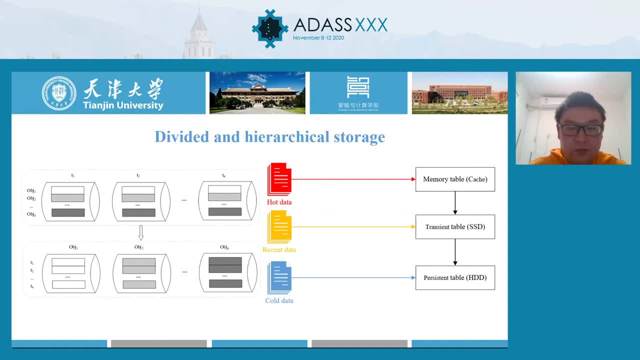 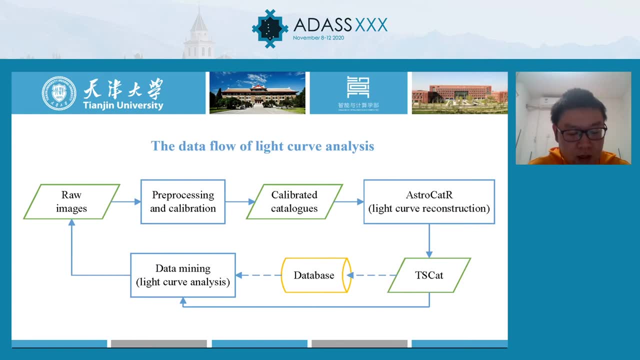 transient table and a persistent table. This figure shows the data flow. of light cover analysis started with raw images. The catalogs are extruded according to the celebration and pre-processing, Then time-series data are reconstructed through astro-coder and exported through TS-CAD storage schema. 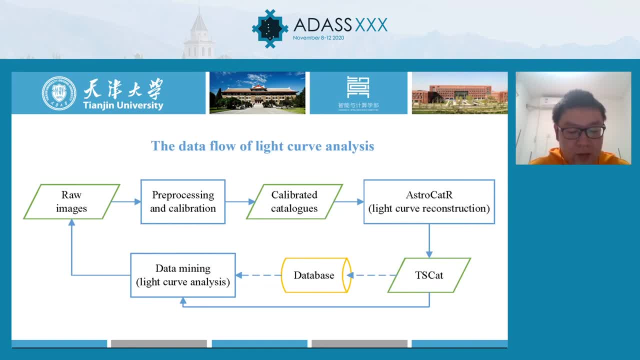 Light cover analysis based on data manner can take advantages of the convenience of databases or directly used in the time-series. This is the case of the time-series data size generated by TS-CAD. The provenance information attached to the TS-CAD can access the sub image for real images. 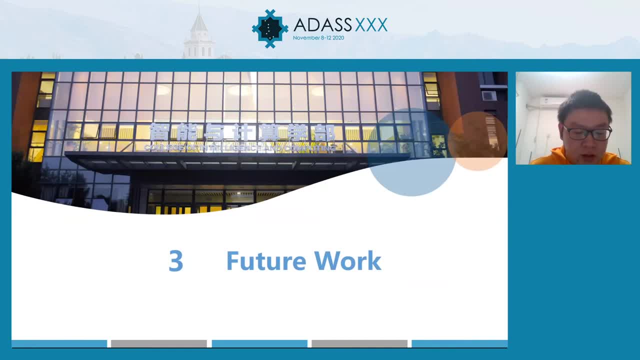 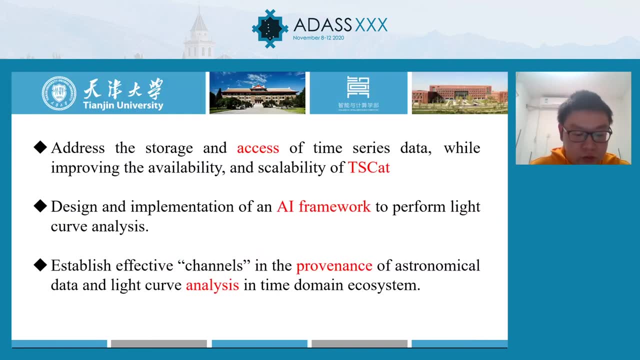 At last I will give you a summary and talk about our future work. I will summarize the the requirements and the challenges of time series storage schema for light cover analysis in time domain, astronomy. we made preliminary design TS-CAT storage schema. For future work we will address storage. 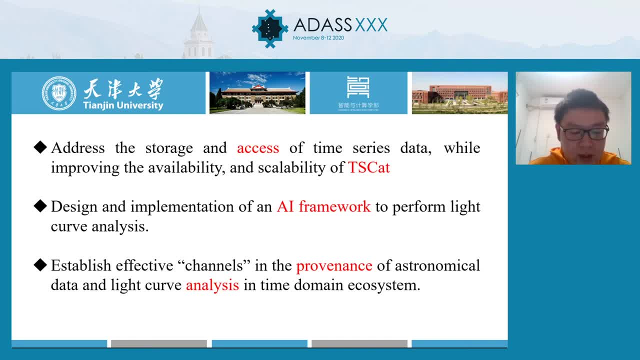 and access of time series data, while improving the availability and scalability of TS-CAT. Furthermore, the framework based on AI techniques will be designed and implemented for light cover analysis. We will try our best to establish effective channels in the provenance of astronomical data. 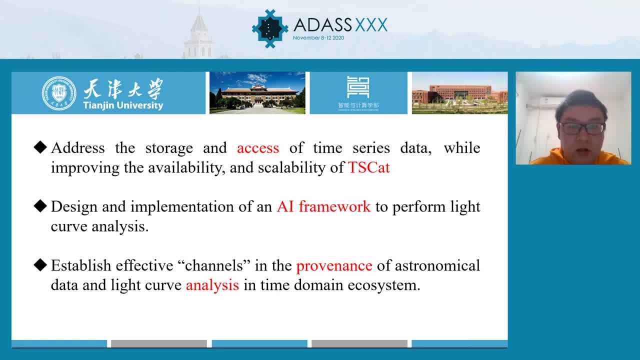 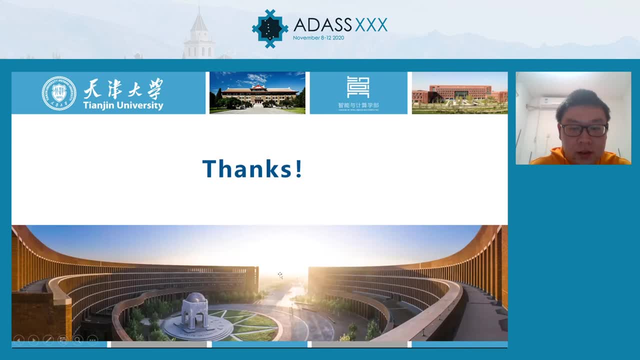 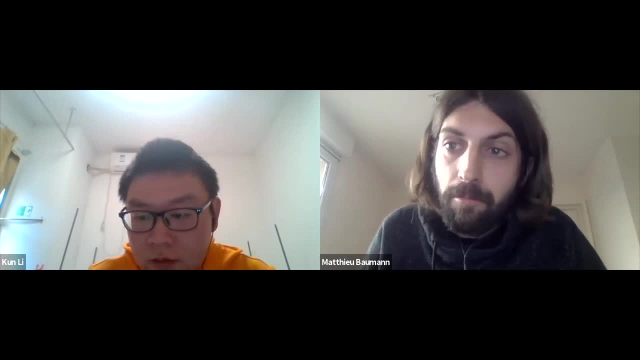 and light cover analysis in time domain ecosystem. Thank you, Fantastic talk. Thank you so much. We have a couple of questions and we have time probably for one or two more. So the first question is: do you plan to use the VIO provenance data model? 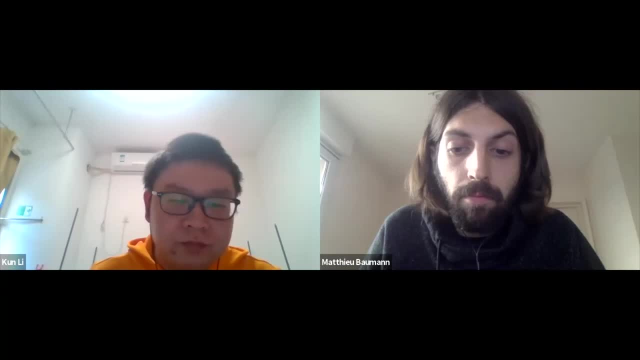 We will. yes, we will. We will use a travel robust tool to make it compatible with VIO provenance data model. Excellent, Thank you very much. Another question: Can this schema be extended to images and not just time series? Maybe currently it's just for catalogs. 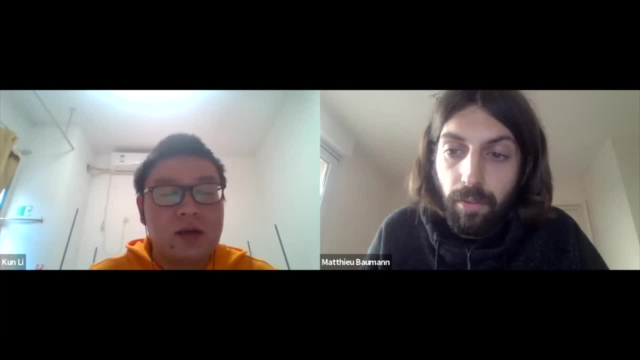 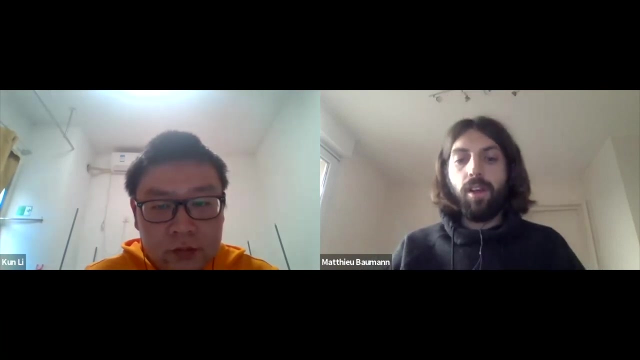 and VIO. We will consider the imager in the future, maybe Fantastic. Another question: can you tell us a little bit about the data volumes and the data rates? The data volume: we adjusted to some experiments using the ASTSAN and the data data. 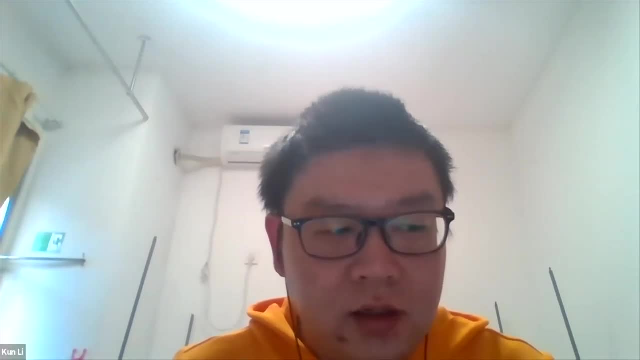 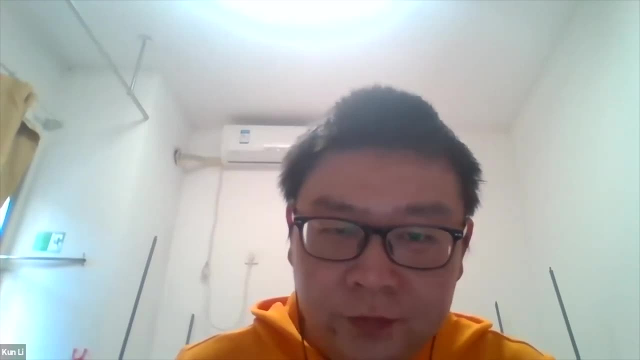 Excellent. thank you very much for your question, for your answers. any other, any other question, otherwise we can also start. oh yes, there is well, Francois is is just commenting that the 2017 idea- a note- was very preliminary, and so that's that's a good thing to keep in mind. yes, I raise documentary. did you look at the 2020 note? 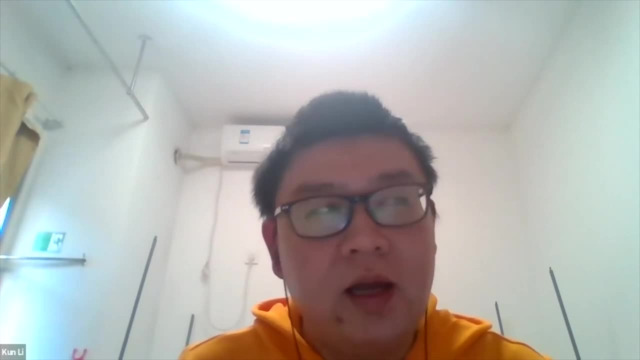 Francois is asking as well: yes, I, I raise astronomy time service. Nick, the documents in 2020, perfect. thank you so much for this great presentation, very interesting.